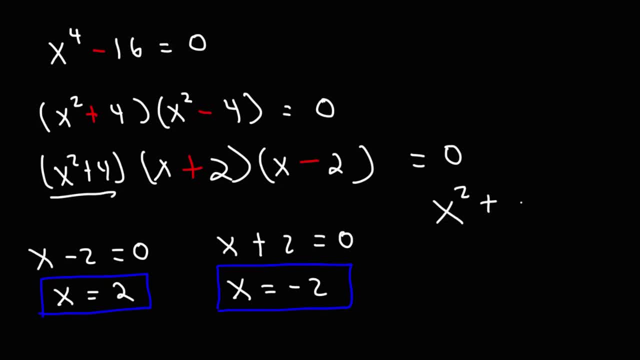 Now let's set this factor equal to 0. What we're going to have to do is subtract both sides by 4.. In doing so, we get this equation: x squared is equal to negative 4.. And then, if we take the square root of both sides, we get that x is equal to plus or minus the square root of negative 4.. 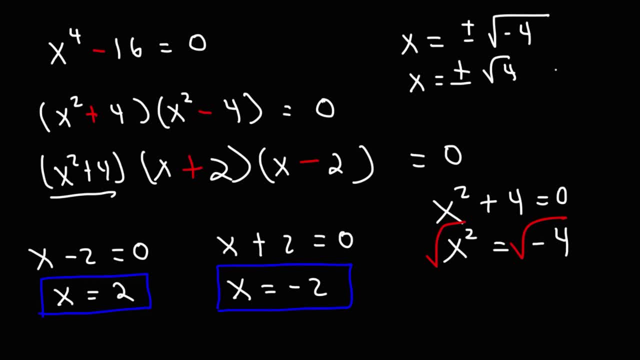 Now we can rewrite the square root of negative 4 as the square root of 4 times the square root of 1.. The square root of 4 is 2.. Now the square root of negative 1 is 2.. The square root of negative 1 is the imaginary number i. 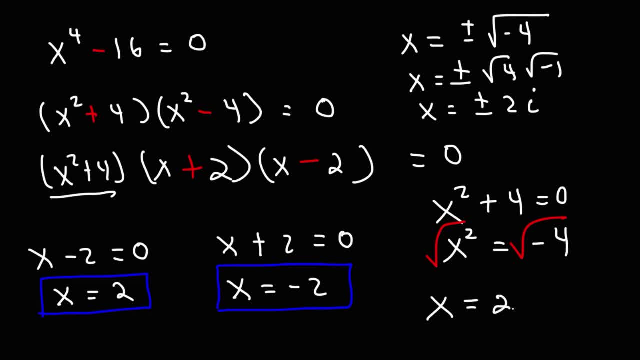 So we get: x is equal to 2i, that is positive 2i, and x is equal to negative 2i. So we get a total of 4 solutions, which makes sense because the degree of the leading term is 4.. 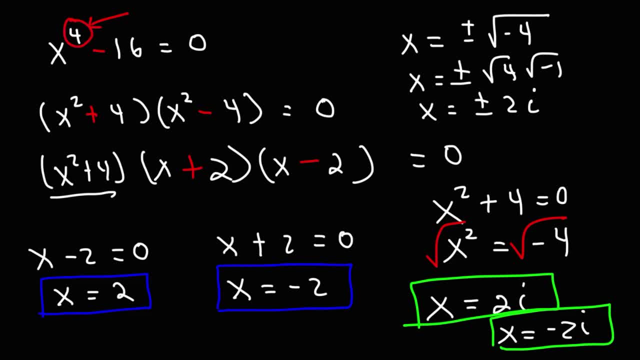 So if the exponent is 4, you can get a maximum of 4 solutions. This includes real solutions and imaginary solutions. In this example, we have 2i. We have 2 real solutions and 2 imaginary solutions, for a total of 4.. 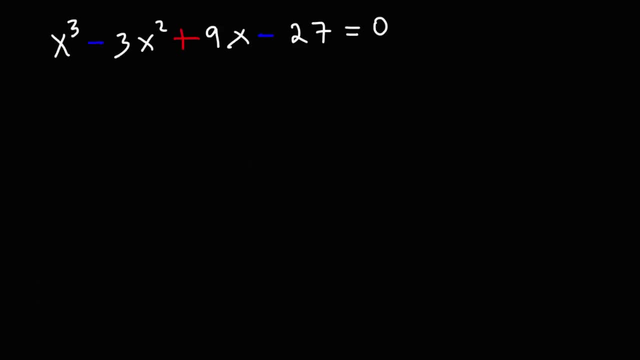 Now let's work on this polynomial function. We have x cubed minus 3x, squared plus 9x minus 27 is equal to 0.. So what are the solutions to this equation? What we can do is we can factor by Grubin. 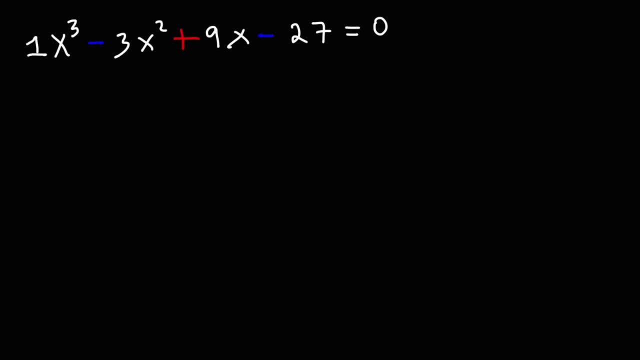 Notice that the ratio of the coefficients of the first two terms is the same as the last two. If we divide negative 4 by 2, we get negative 4.. If we divide negative 3 by 1, we're going to get negative 3.. 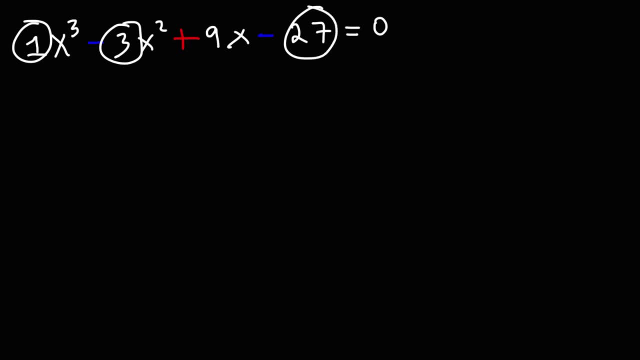 If we divide negative 27 by 9, we will also get negative 3.. When you see that, you can factor by Grubin. So let's take out the GCF in the first two terms. The greatest common factor is x squared. 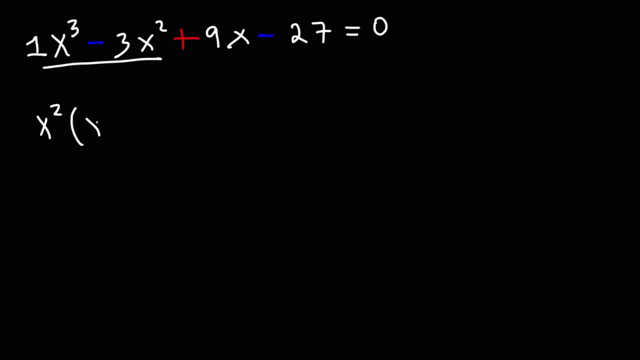 If we divide x cubed by x squared, we're going to get x. And if we divide negative 3x squared by x squared, we're going to get negative 3.. Now let's do the same thing for the last two terms. 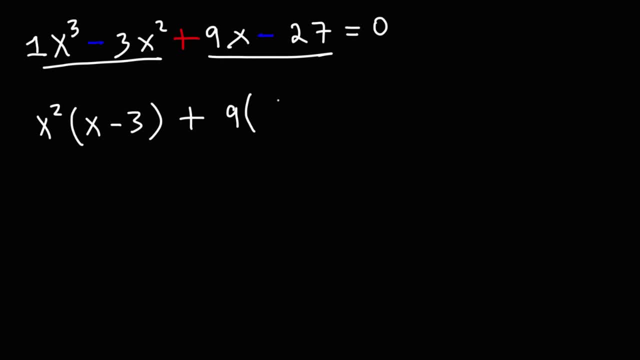 The GCF is 9.. 9x divided by 9 is x Negative. 27 divided by 9 is negative 3.. So note that we have these two common factors. If they're the same, you know you're on the right track. 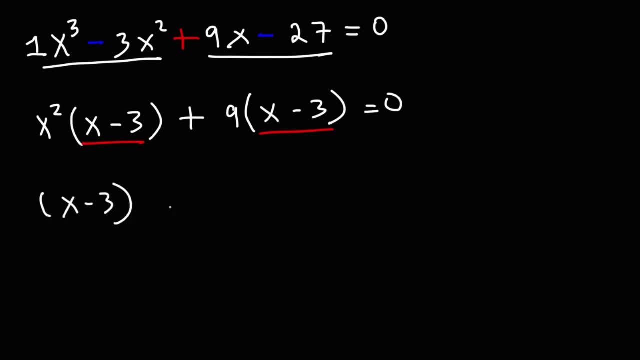 So we're going to factor out x minus 3.. If we take away x minus 3 from the first term, we're left with x squared, And if we take away x minus 3 from the second term, we're left with plus 9.. 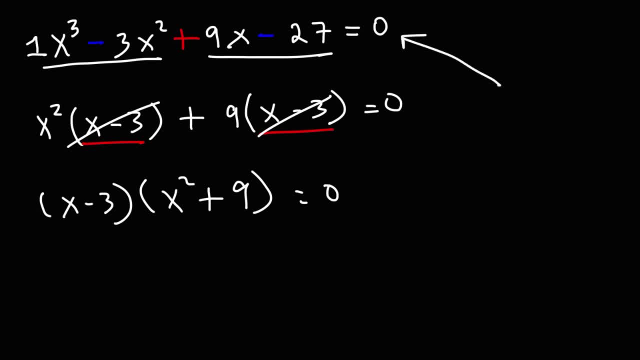 So this is how we can factor the original equation. Now let's set each factor equal to 0.. For the first one, we just need to add 3 to both sides and we get the solution: x is equal to 3.. For the second one, we need to subtract both sides by 9.. 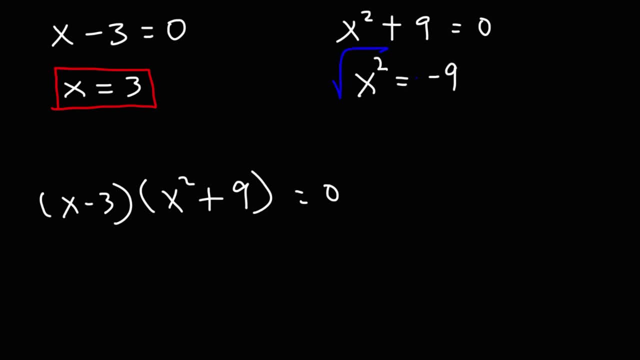 We're going to get: x is equal to, or rather x squared is equal to, negative 9.. Taking the square root of both sides, we get that x is equal to plus or minus the square root of negative 9.. Which we can break it up into the square root of 9 times the square root of negative 1.. 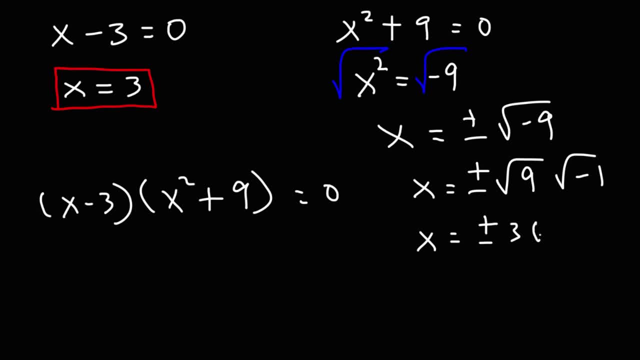 The square root of 9 is 3.. The square root of negative 1 is i. So we have a total of three solutions because our original problem was a degree 3 polynomial. So we have one real solution And we have two imaginary solutions for a total of three solutions. 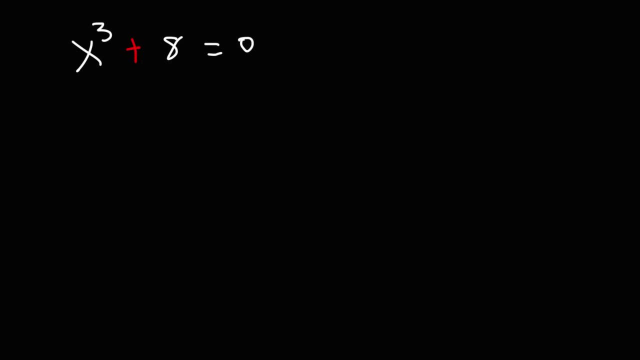 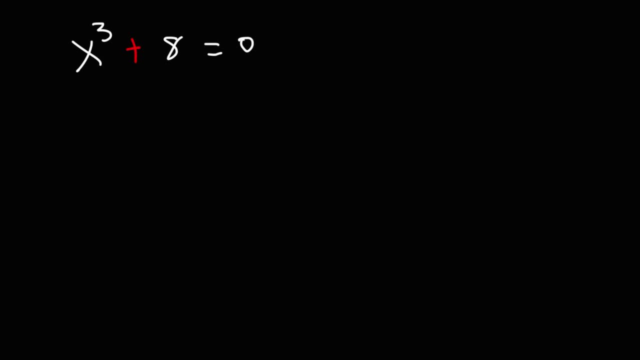 might get one real solution and two imaginary solutions, But let's find out. So what we have is a sum of perfect cubes. So we could use this formula: a to the third plus b to the third can be factored into a plus b times a squared minus ab plus b squared. 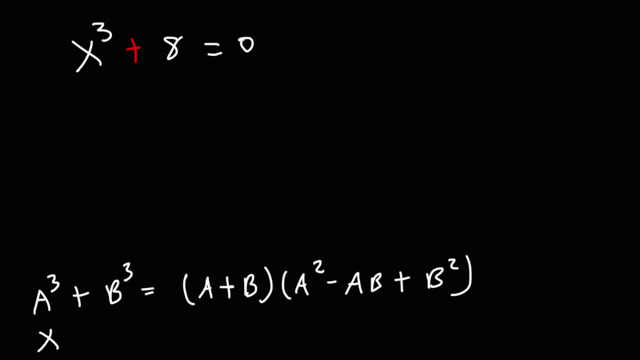 So x cubed is a cubed, b to the third is eight. a is going to be the cube root of x cubed, which is x. b is going to be the cube root of eight, which is two. a squared is going to be x squared, and. 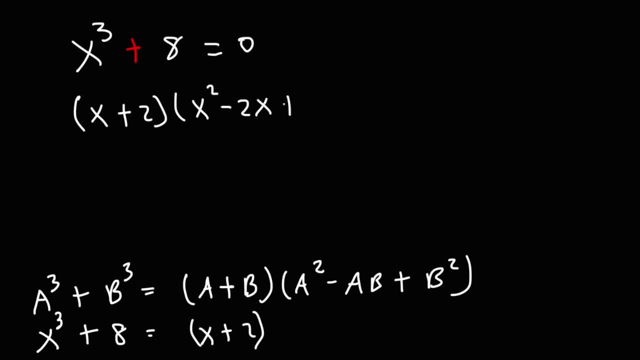 then a times b, that's two times x, with a negative sign, and then b squared or two squared, which is four, And so we get this. Now let's set each factor equal to zero. Subtracting both sides by two, we get our first answer: x is equal to negative two. For the second one, we need to use the quadratic formula. 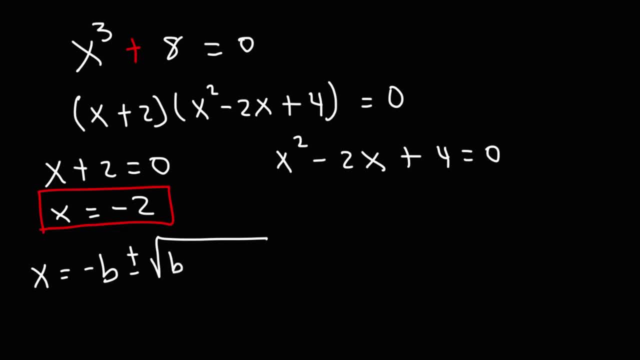 x is equal to negative. b plus or minus. the square root of b squared minus four ac over two a. a is the number of times b squared minus four ac over two a. a is the number of times b squared minus four ac over two a. 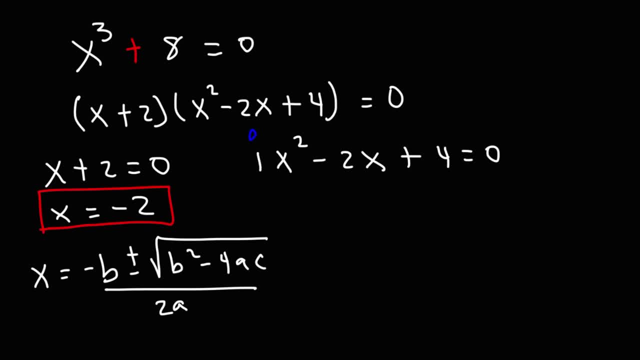 b is the number in front of x squared. b is the number in front of x. c is the constant term. So this is going to be negative negative two plus or minus. the square root of negative two squared minus four, ac over two. a and a is one. 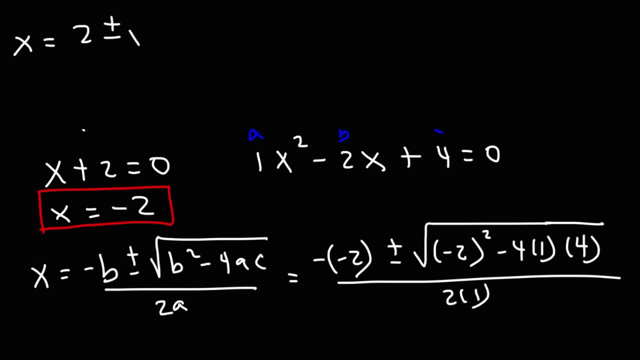 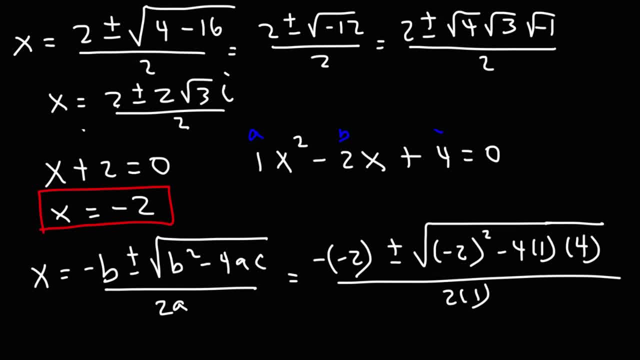 negative. 1 is i. So we get this, And then we could divide each of these numbers by the denominator of 2.. So we get that x is going to be 1 plus or minus 1, square root 3i or simply square root 3i. So we have a total of 3 solutions. We have 1 real solution and 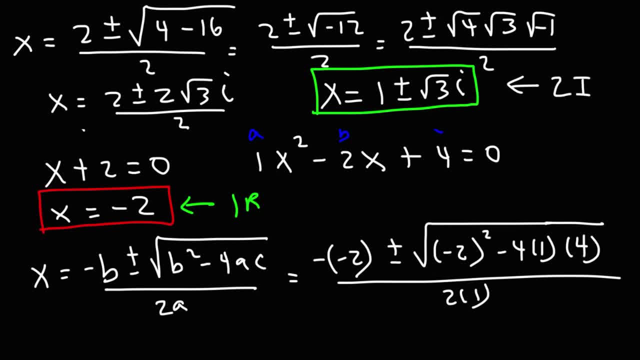 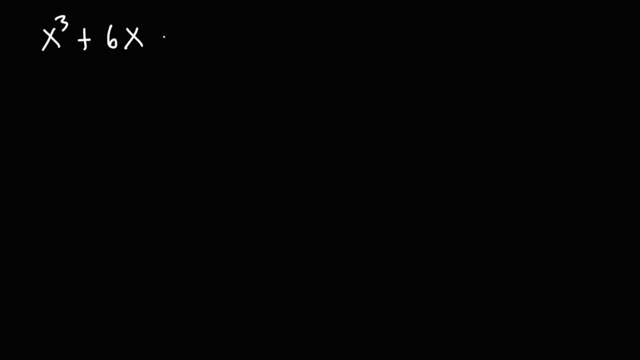 here we have 2 imaginary solutions. The first imaginary solution is 1 plus root 3i. The second is 1 minus the square root of 3 times i. Now let's work on one more example. So let's say we have the polynomial function: x cubed plus 6x minus 7 is equal to 0. How 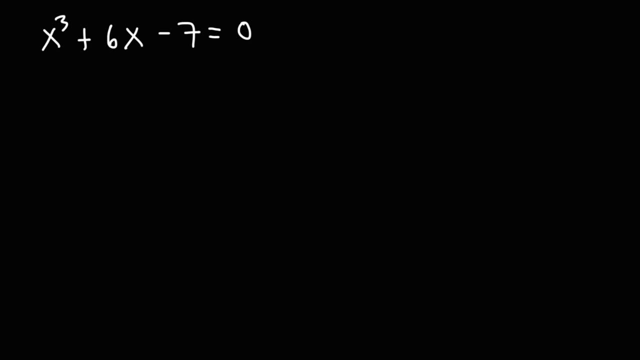 can we solve this one? Well, it's going to be hard to factor this expression, but we could use syntax. Before we do that, we need to make a list of all the possible zeros that might work for this function. To do that, take all the factors of the constant term 7.. So that would 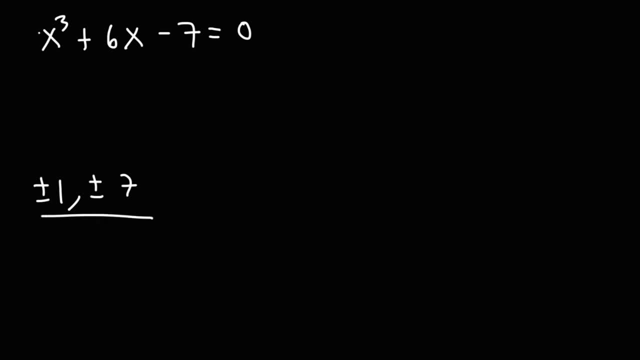 be plus or minus 1, plus or minus 7.. And then write down the factors of the leading coefficient in front of the highest term. So the factors of 1 is just plus or minus 1.. So when we divide this we get just 1 and 7.. Let's try positive 1.. 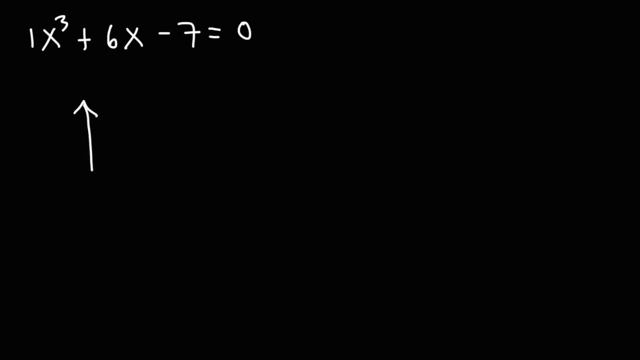 Let's see if that works. So we're going to use synthetic division And we're going to write the coefficients of this equation. So we have 1x cubed, so we're going to write 1.. Now we don't have an x squared, so you could think of it as plus 0x squared And 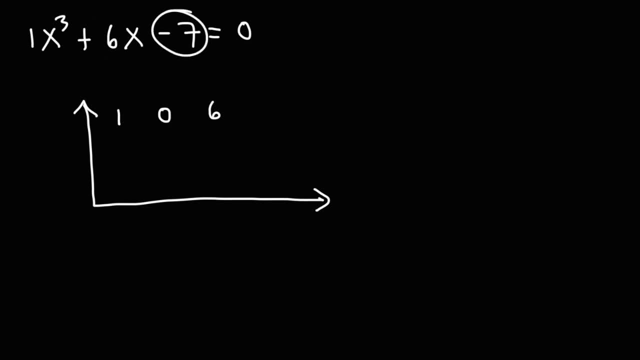 then it's plus 6x minus 7.. And then we're trying: x equals 1.. So we're going to put this number there. Let's bring down the 1.. We need to multiply these two numbers. 1 times 1 is 1.. And then we're going to add these: 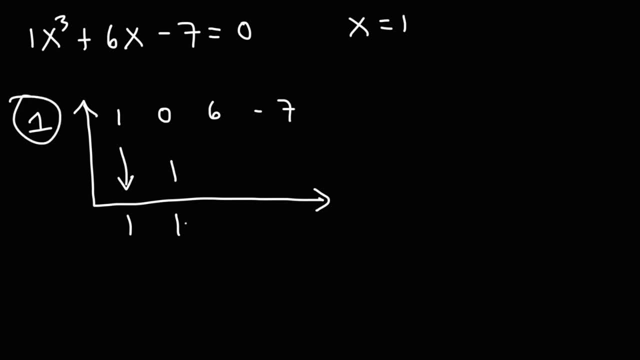 two numbers: 0 plus 1 is 1.. And then multiply 1 times 1 is 1.. And then add: 6 plus 1 is 7.. 1 times 7 is 7.. And then negative: 7 plus 7 is 0. If you get a 0, that means it works. 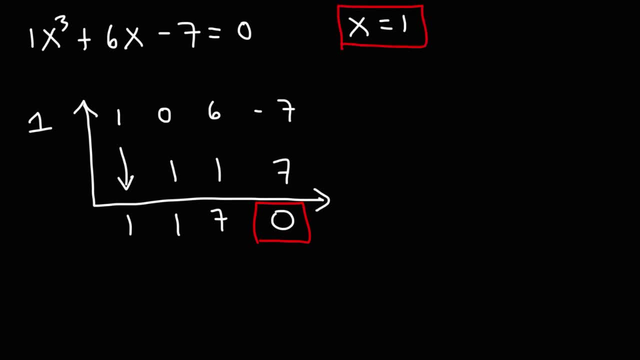 It means that 1 is a solution. If you were to plug in 1 into this equation, you would get 0.. 1 to the 3rd plus 6 times 1 minus 7, that's equal to 0.. 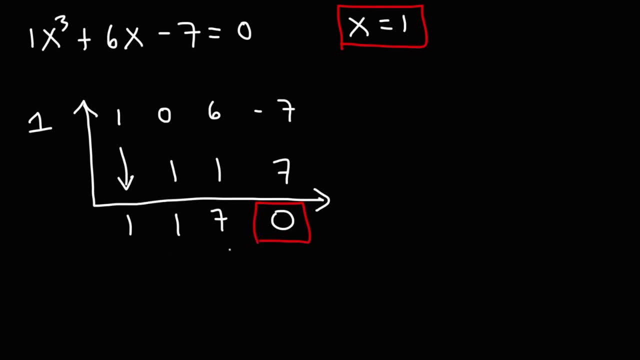 Now let's turn this into a factor. This is the constant term 7. This is the number in front of x And this is the number in front of x squared. So thus we can rewrite the equation in its factored form like this: 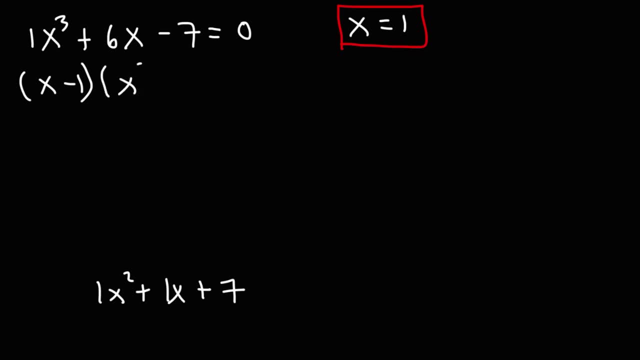 Which comes from this solution: Times x squared plus x plus 7.. So we already have the solution for this factor. We need the solution for this one. So we need to use the quadratic equation So we can see that a is 1,, b is 1, and c is 7.. 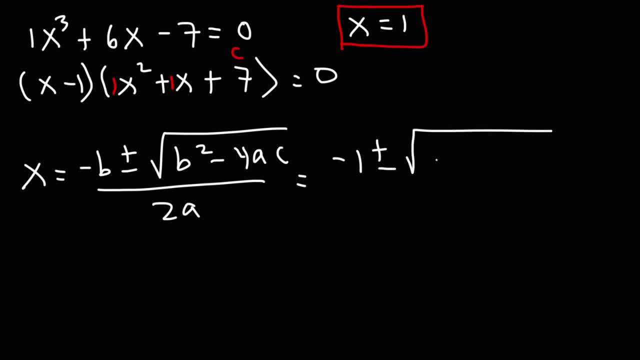 So it's going to be negative 1 plus or minus the square root of 1 squared minus 4 times 1 times 7 over 2.. Or 2 times 1.. So this is going to be 1 minus 28,, which is negative 27.. 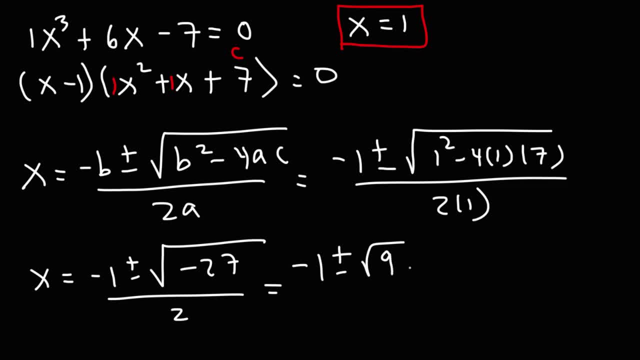 Now negative 27,. we can write that as the square root of 9 times the square root of 3 times the square root of negative 1.. The square root of 9 is 3.. And we can replace the square root of negative 1 with i. 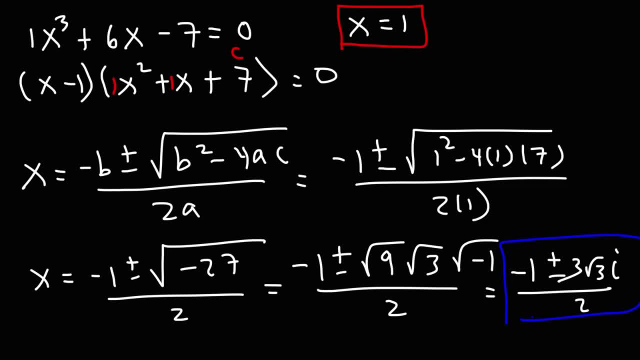 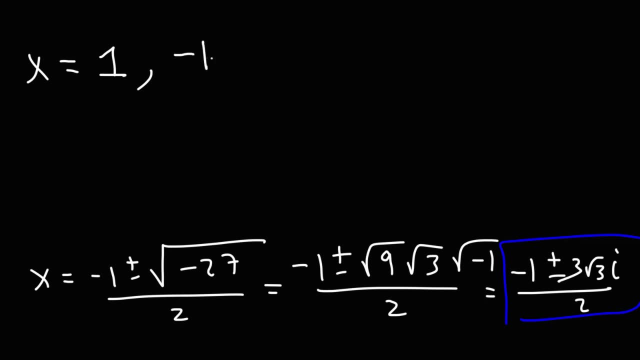 And so this is the solution. So let's write out each individual solution. So we have one real solution that is x is equal to 1.. And then we have two imaginary solutions. The first one is going to be negative, 1 plus. 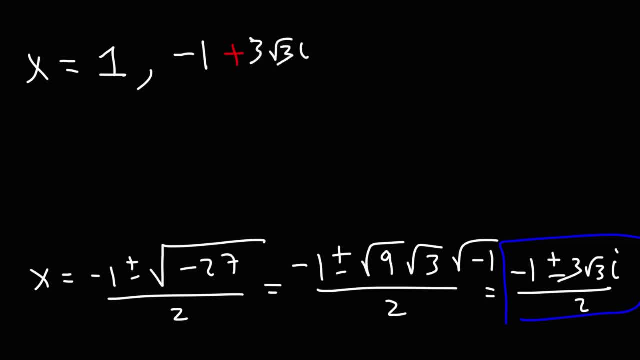 3 root 3 times i, divided by 2.. The second one is going to be negative: 1 minus 3 root 3 times i over 2.. So those are the three solutions that we have for this polynomial equation.